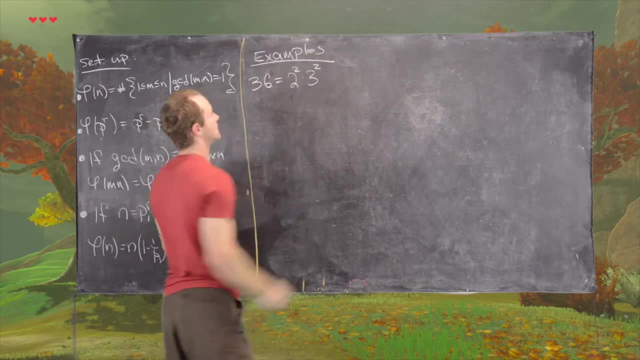 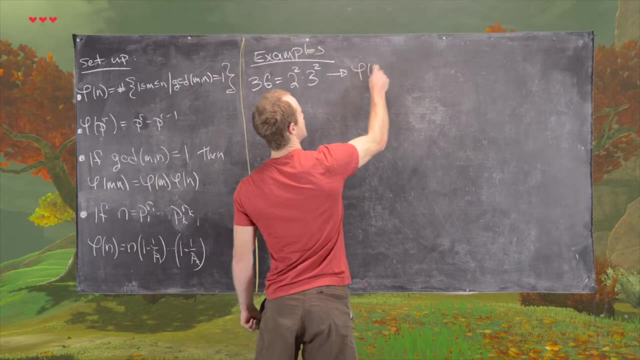 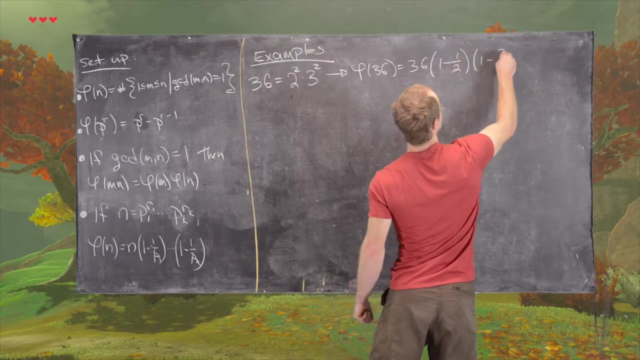 And so that's easy because we can write down its prime factorization very quickly. So it's 2 squared times 3 squared, And so that tells us that phi of 36 equals 36 times 1 minus half, and then 1 minus 2 thirds. 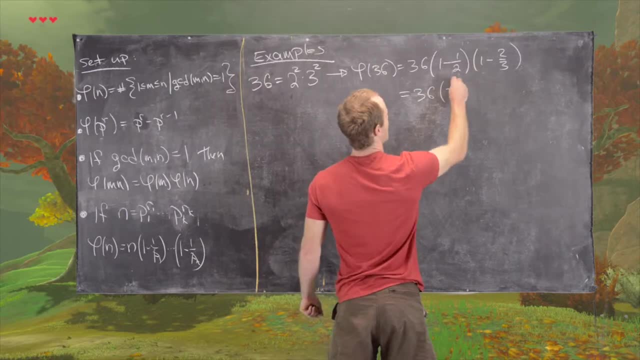 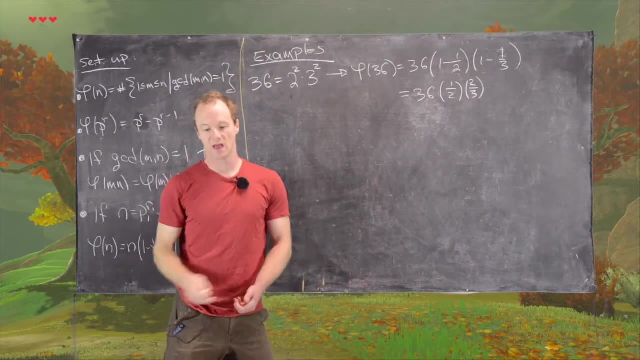 So that's going to be 36 times 1, half times 2 thirds. Sorry, that should be 1 third. I was getting ahead of myself. Good, And then, as you can see, we can cancel that, And then 36 over 3 is 12.. 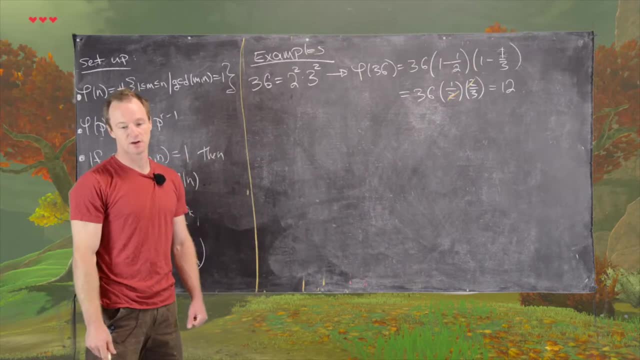 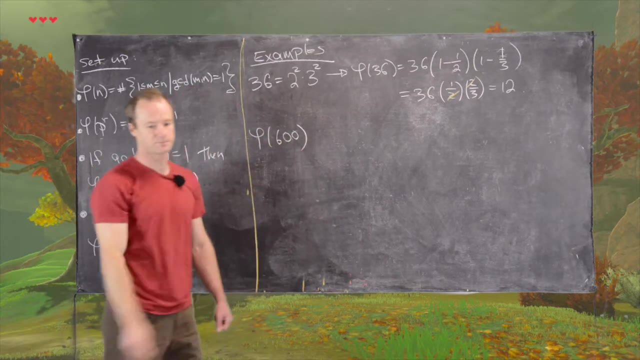 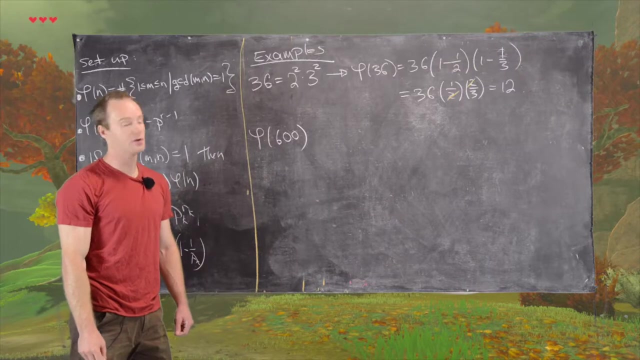 So we have: phi of 36 is 12.. Good, So let's look at another example. So maybe phi of 600.. So The prime factors of 600 are only 2,, 3, and 5. So I'll let you check that. 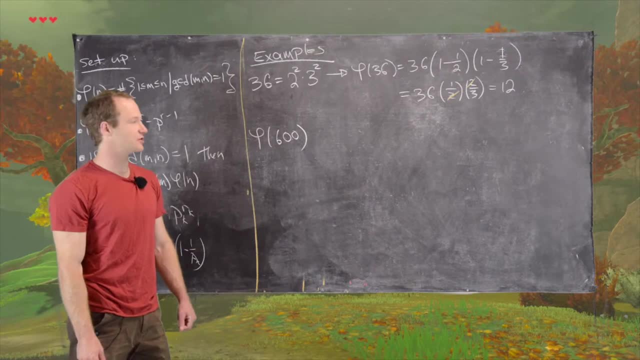 And I won't even write down what exponents we need for 2,, 3, and 5.. I'll just use the fact that we have this formula. So 2,, 3, and 5 are the only prime factors here. 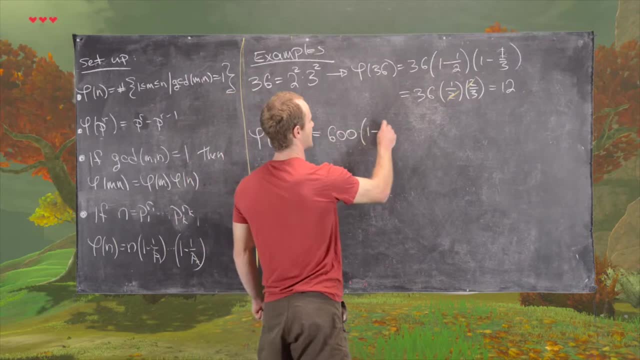 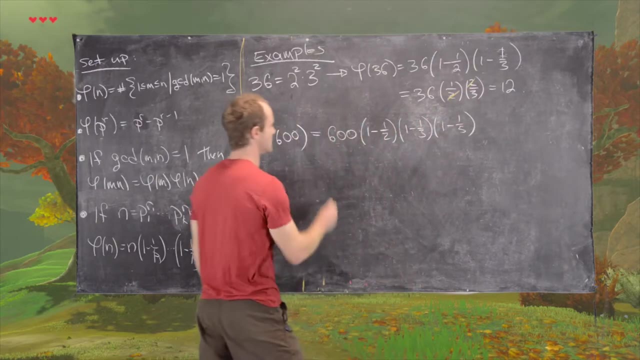 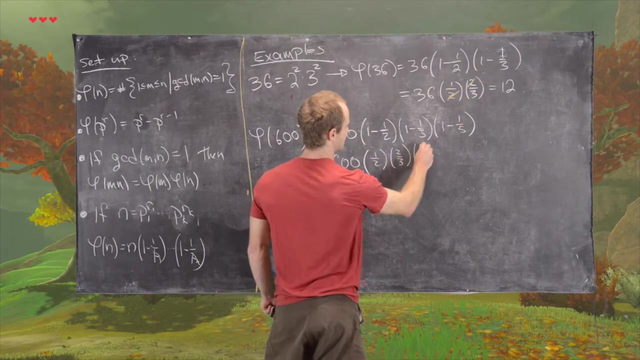 So that means this is going to be 600 times 1 minus half times 1 minus third times 1 minus fifth. Good, So that will be 600.. And then 1 half times 2 thirds times 4, fifths- Great. 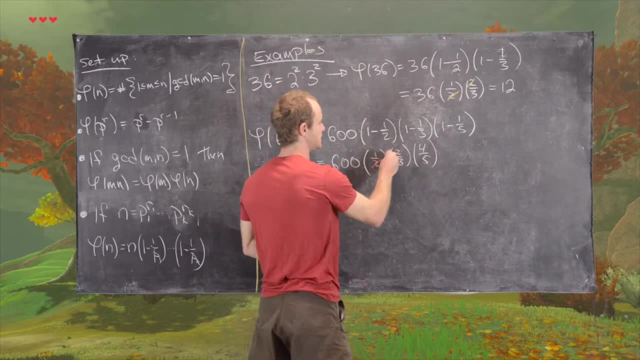 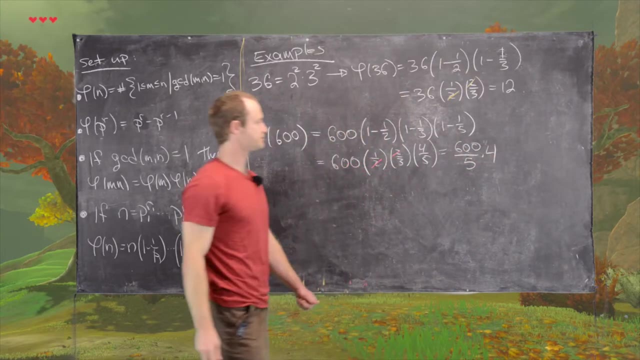 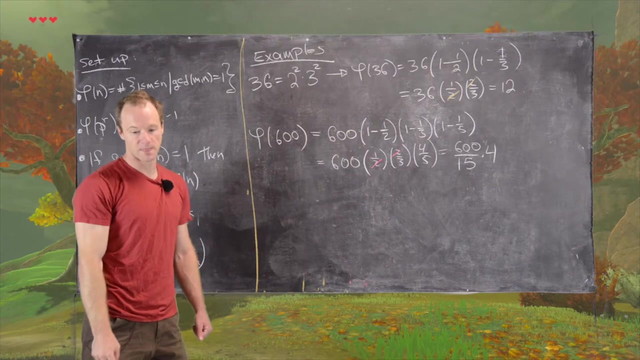 So let's see what we can get from that. So these 2s cancel And we're left with 600 over 5 times 4.. Sorry, maybe 600 over 15 times 4.. And then we can check that. 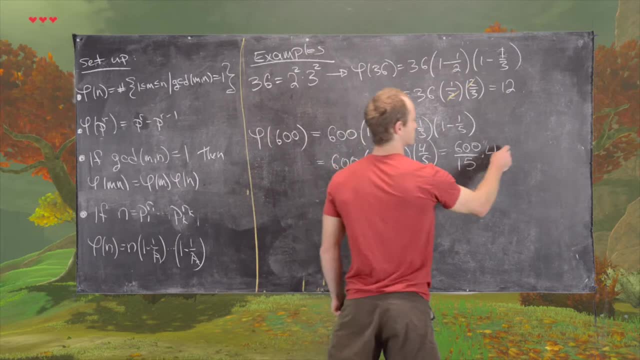 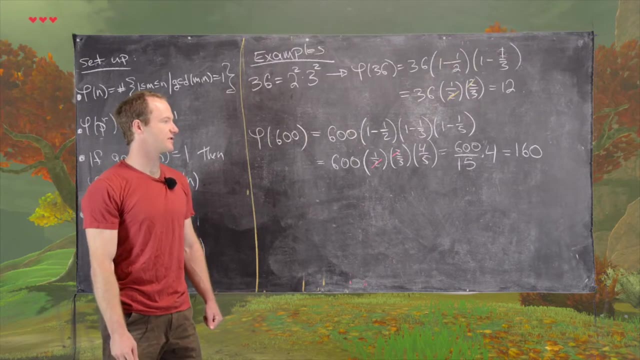 But this is equal to 160.. So this is equal to 160.. So it's maybe easy to check that 600 divided by 5 is 120.. And then divided by another 3 is 40. And then multiplied by 4 is 160. 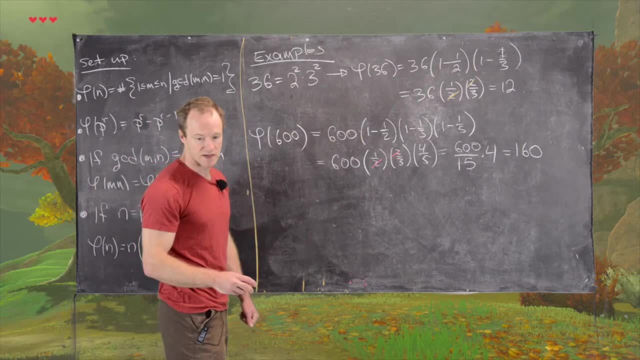 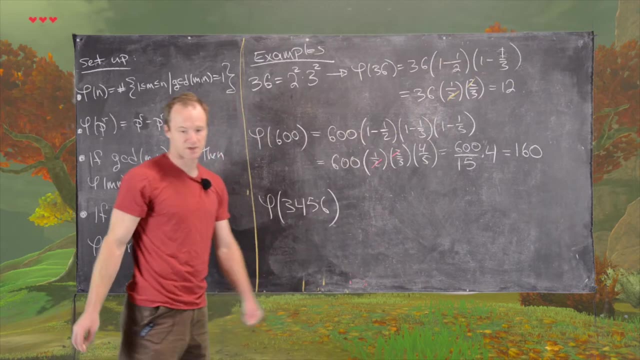 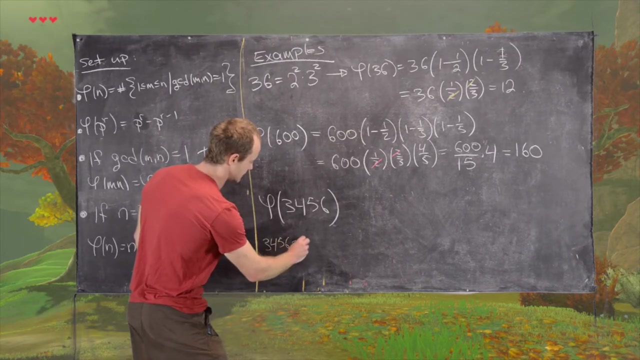 Good, So let's do maybe one more example. So let's maybe do phi of 3,, 4,, 5,, 6.. And so in this case we'll use the fact that this 3, 4,, 5, 6 is equal to 2 to the 7 times 3 squared.